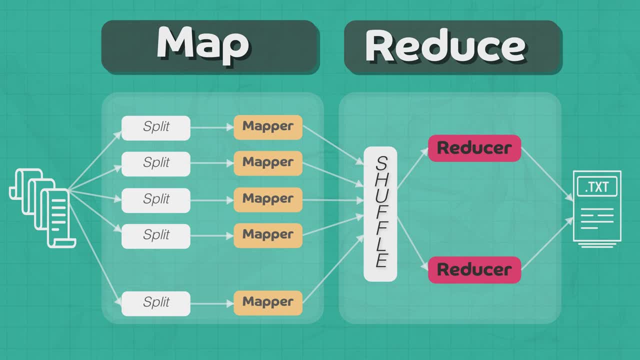 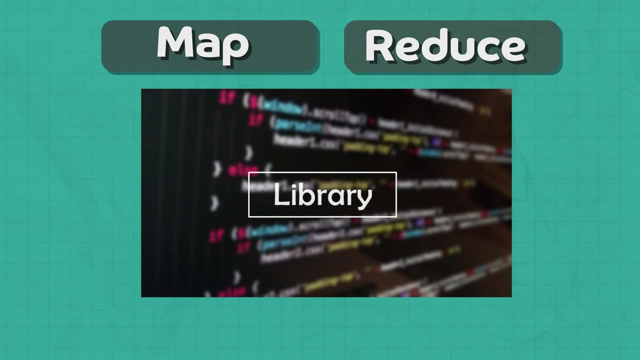 functions Here in the context of MapReduce. in distributed system settings, Map and Reduce are a little bit different. Google engineers realized that most of the data processing tasks could be split up into two steps, and they created a library that allowed engineers to process huge datasets. 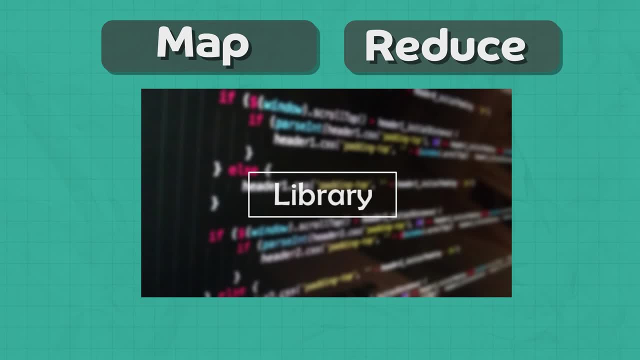 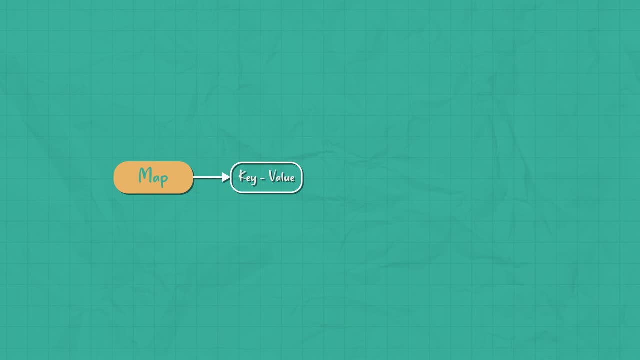 in order of terabytes spread across thousands of machines, And this is a fairly simple concept to understand. There is this map function that transforms the data into key-value pairs. The key-value pairs are shuffled around and reorganized. they are then reduced to some. 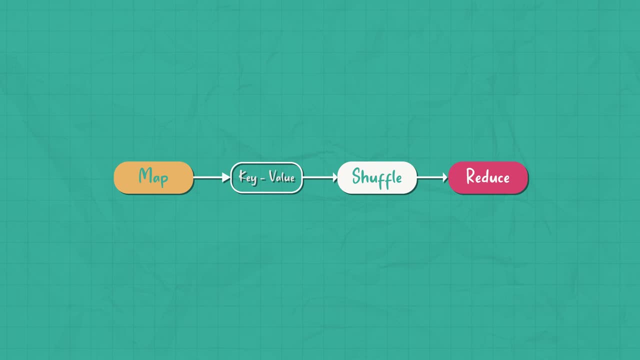 final output. Now, before understanding it any further through an example, there are a few things worth noting. The first thing is that when dealing with MapReduce model, we assume that we have a distributed file system, Which means we have got some large datasets that are split up into chunks. 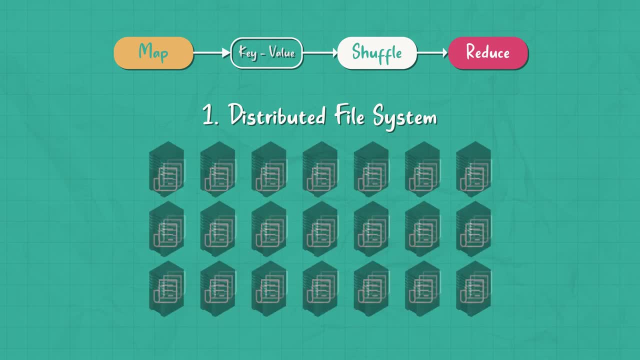 These chunks are replicated and spread out across hundreds of thousands of machines, and then This distributed file system has some sort of central controller which is aware of everything going on in the MapReduce job, Meaning the central controller will know where exactly the chunks of data resides and is. 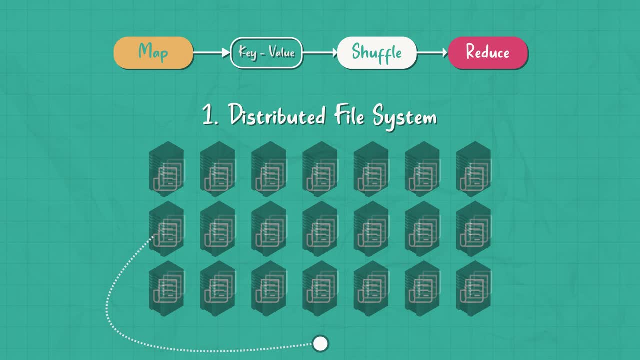 able to communicate with all the machines that store or process this data, That is, the Map machines or Reduce machines or workers. The second thing to note is that, since we are dealing with very large datasets, we don't actually want to move these large datasets. 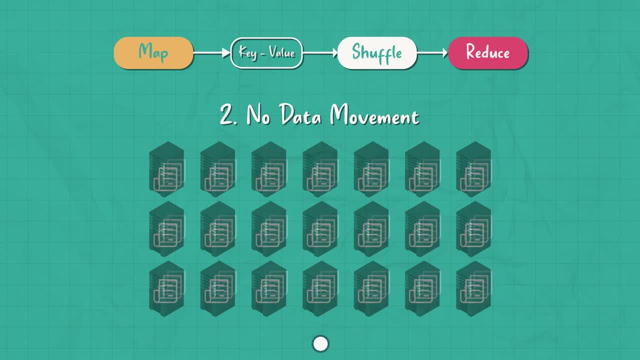 We let them live where they currently live on their respective machines. What we do is we have these map functions operate to the data locally. So instead of grabbing and aggregating the data and move it somewhere else, we instead send the map programs to the data and avoid moving all this large data. 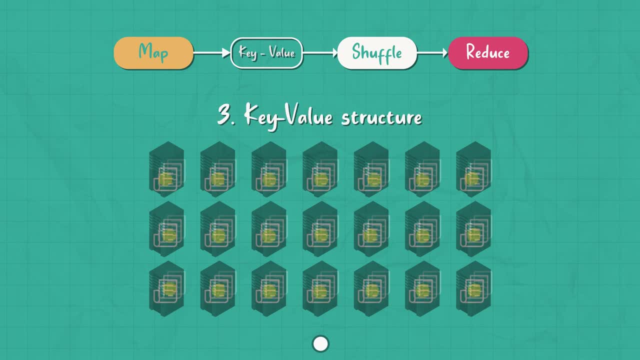 The third very important thing to note about this model is the key value structure of data in the intermediary step is very important Because when you perform a reduce or reduce data chunks, these data chunks come from the same dataset Because, remember, Most of these data chunks are the chunks of the same large dataset. 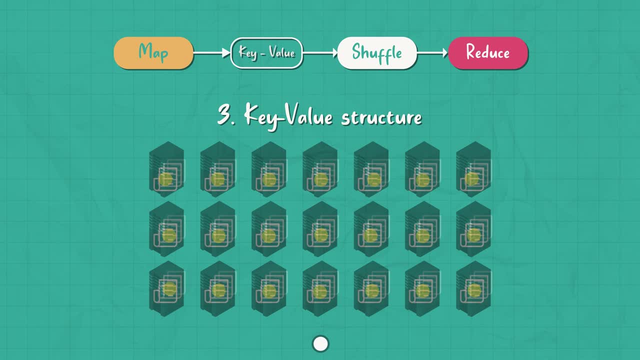 So when you reduce these data chunks, you are likely looking into some sort of commonality or pattern in these various pieces of data, Because when you got key value pairs, you will have some keys that are common, Some keys that are common up here, some keys that are common up here or down here, and it 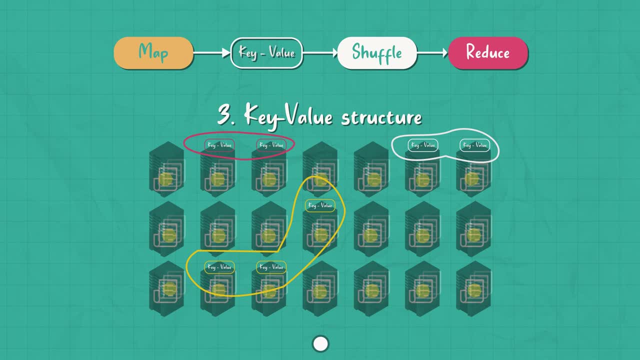 becomes easy to reduce them into one single meaningful value based on that key. This will become very clear when we deep dive into our example. The fourth thing to note is how the model has to work To handle machine failures or network partition. To handle failures, the MapReduce model basically re-performs the map operations or the reduce. 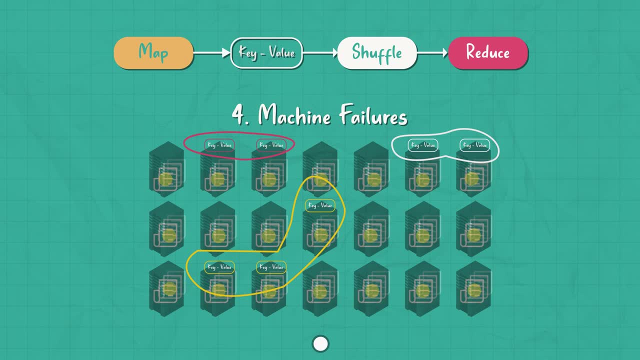 operations when the failures occurs. So if a failure occurs in the step here, that is, maybe there was a network partition when generating the key value pair, The central controller, which I mentioned earlier, will just re-perform this operation and then move on to the reduce step. 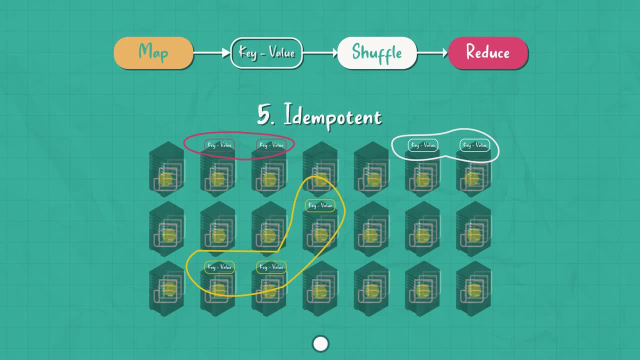 And this can happen only if the map and reduce functions are idempotent. that is, if we repeat the map or reduce function multiple times, The output doesn't change. The outcome doesn't change regardless of how many times we repeat the map or reduce. 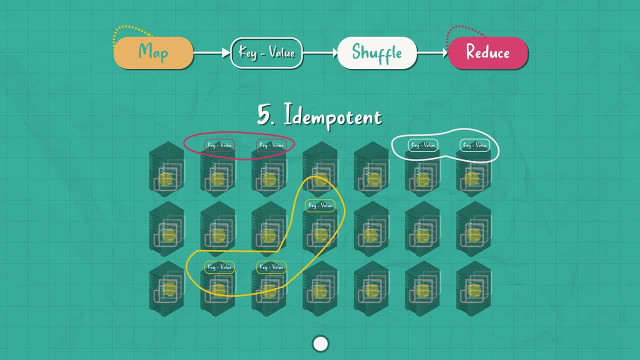 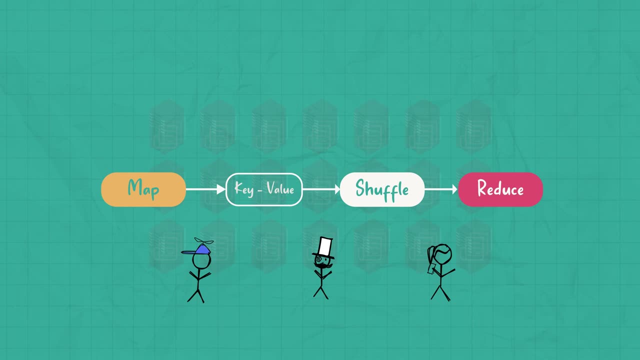 function. So idempotency is a requirement in the MapReduce model. Now, when engineers are dealing with the MapReduce model, they just need to make sure that they have a good understanding of the inputs and expected output. That is what is the output of the map function. what is the intermediary key value pairs- look, 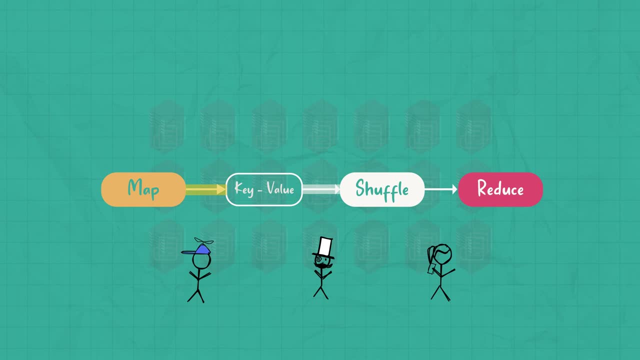 like how they can be reorganized in a meaningful way which, as an input to the, reduce function and allow it to optimally work. As you can see, this framework simplifies a lot of things for engineers. Engineers just need to worry about the input and output data in various steps. 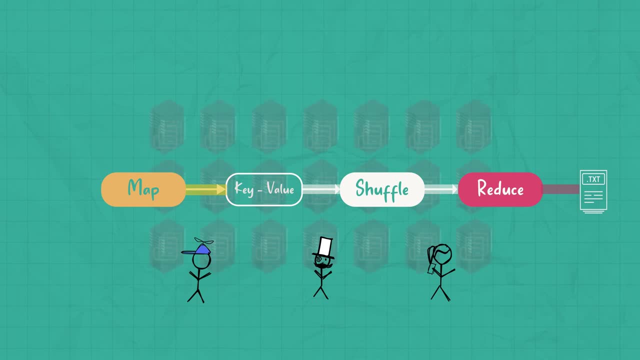 They don't need to worry about the intricacies and complexities of processing large datasets in a distributed system. Basically, engineers will end up using some sort of library implementation, such as Hadoop, and they just need to be aware of the various inputs and outputs of these various functions. 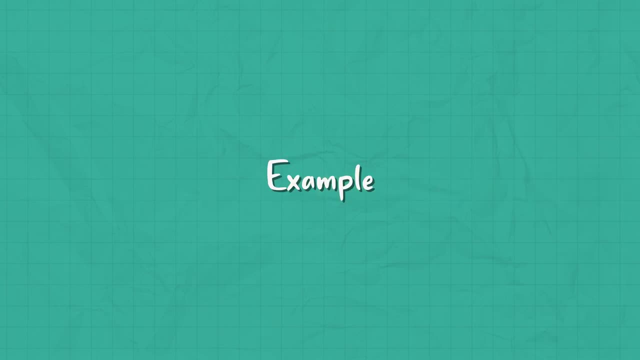 Alright, With all these points in mind, let's understand it through an example which I am taking from the same white paper presented by the Google engineers. So here I have a set of input files, and typically these input files will be distributed across. 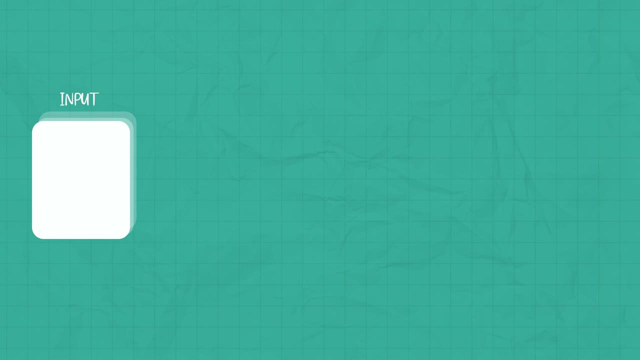 several machines. For our example, for the sake of simplicity, I just have two input files, And our task here is to count the number of occurrences of each unique word across all the files. So here, our first file contains the sentence this is an apple, and our second file contains: 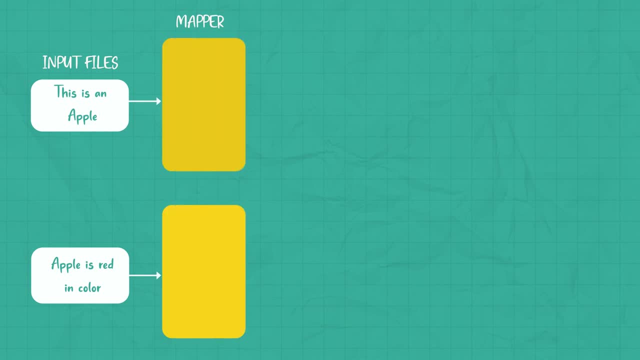 apple is red in color. The mapper here counts the number of times each word occurs from the input splits in the form of key-value pairs, where the key will be the word and the value is the frequency of the word, So the word this occurs one time. the word is occurs one time the word an apple is one. 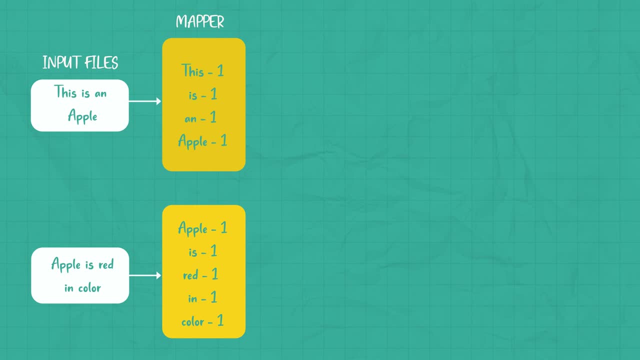 time and the word apple occurs one time. And same with the other input file where it says apple is red in color. the word apple occurs one time, is occurs one time, red occurs one time, in occurs one time and color occurs. 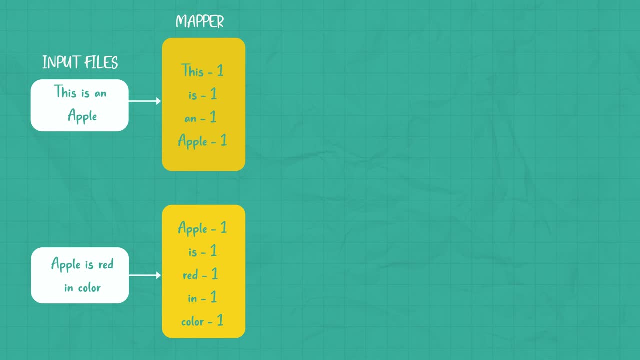 one time. By the way, both these operations, both the mapping operations, are happening here in parallel. Now, once the mapping is done, it is followed by a shuffle phase, which is a lot of times ignored during the MapReduce discussions, but it's a critical step. 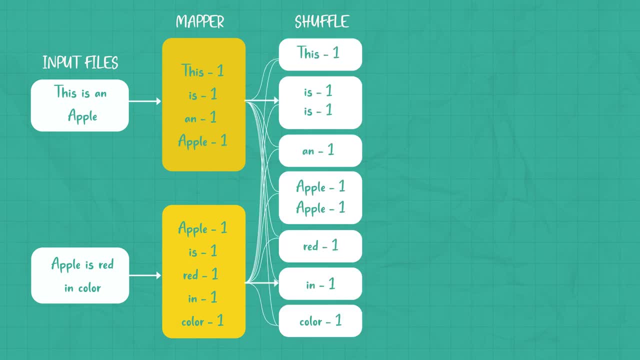 Here we group the values by keys, in the form of key-value pairs. So here we got a total of six groups of key-value pairs, And these shuffling or grouping of keys makes the job of reducer so easy and efficient, Because now the same thing happens. 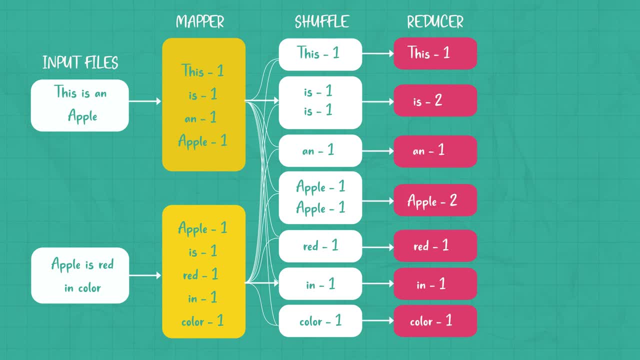 Now the same reducer is used for the same key-value pairs with the same key. Now all the words present in the data are combined into a single output in the reducer phase And the output shows the frequency of each word. Here in the example we get the final output of key-value pairs, as this occurred one time. 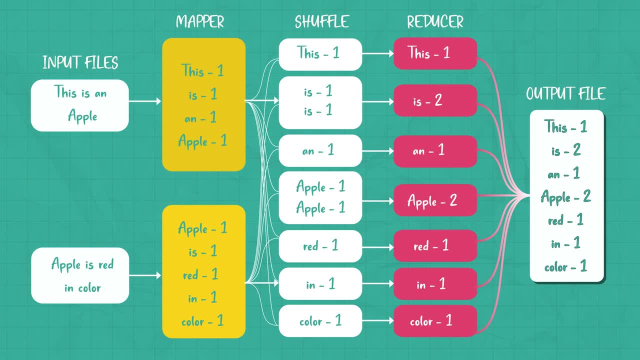 the word is occurred two times: an occurred one time, apple occurred two times, red occurred one time, in occurred one time, and color occurred one time. The trickier part in the context of system design interviews is to be able to identify this pattern of MapReduce that is given a problem. can you solve that problem using? 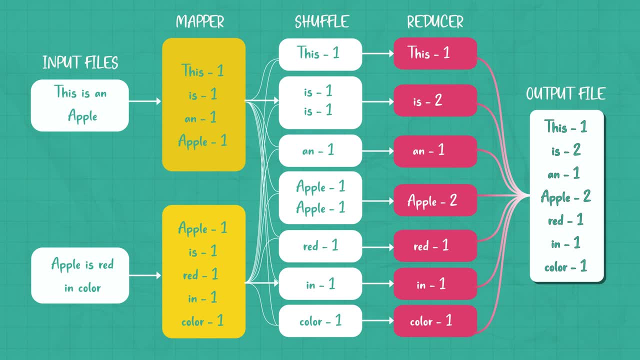 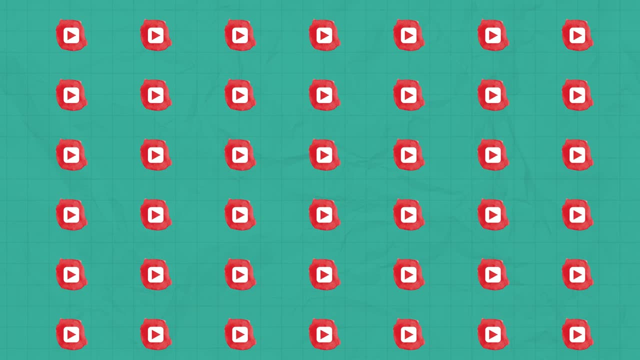 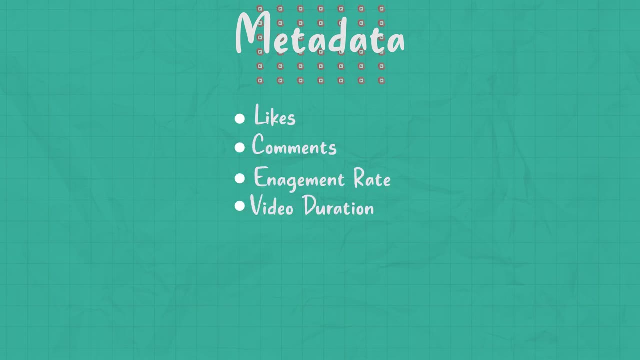 MapReduce. Is that the real use case? So that is something you need to be able to identify and which comes by solving more and more problems. So, for example, you are given a large data set of millions of YouTube videos and their metadata information, such as the likes, the comments, the engagement rate, the length. 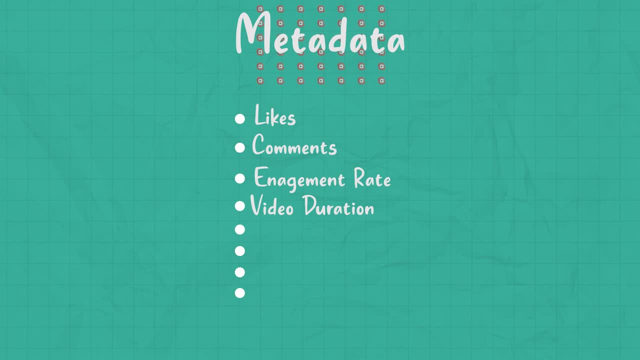 of the video and whatnot. And let's say, you are asked to find all the videos which have certain number of likes. So for this, you need to find all the videos which have certain number of likes. So for this, you need to find all the videos which have certain number of likes. 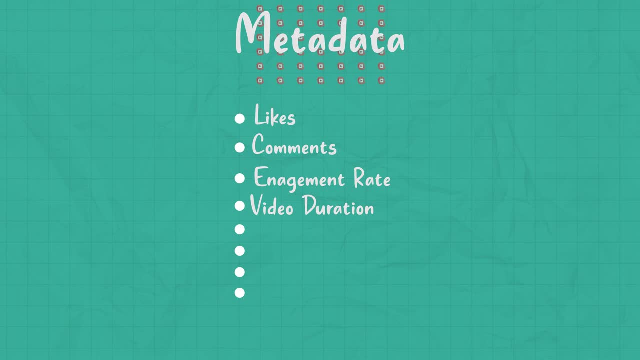 So for this you need to find all the videos which have certain number of likes, You need to parse through the entire metadata information of all these videos and then finally produce an output file. and likewise, whenever you are given a large data set where you have to deduce or analyze the large data set, where, say, the files are distributed across.